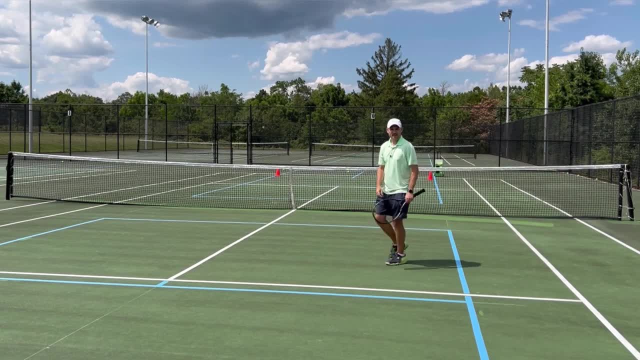 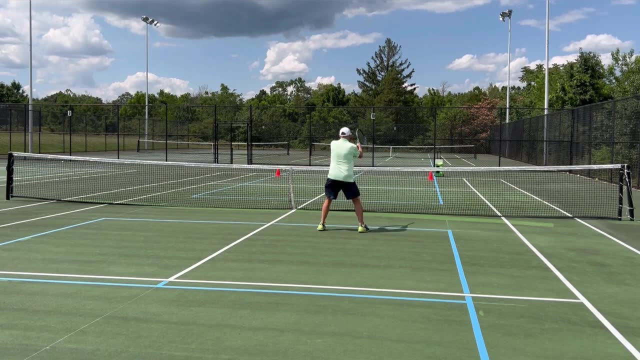 up. your opponent can run that down and then pass you down the line. You're better off keeping the ball in front of you, which means you keep your opponent in front of you And that way you don't have to go as far to bisect, where they can hit the ball On this side if they go for. 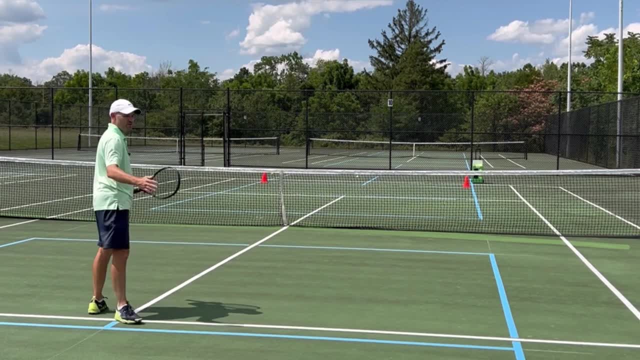 a high volley, they're going to hit the ball. If they hit a low volley, they're going to hit the cross court pass. and I have a low backhand. it's the exact same thing. Low volley should be hit in front of you. I will say this because I'm sure someone's typing right now. If the ball is in the 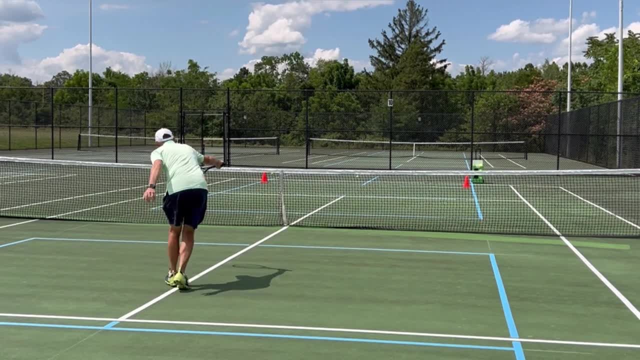 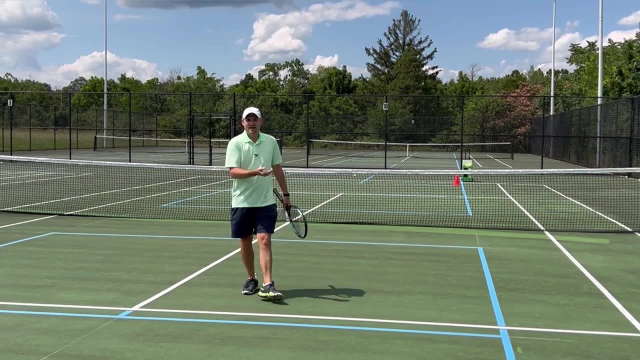 middle. it doesn't matter which cone you aim for. Move the low volley that's in the middle to a cone. Obviously, you'll move to that side and then you'll bisect. All right, watch me hit some low volleys and I'm going to try to hit the cone that's in front of me. All right, here we go. 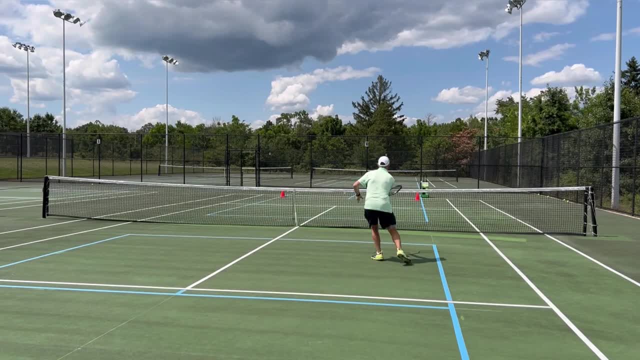 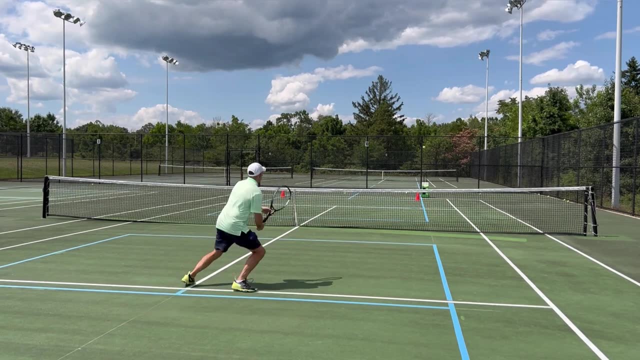 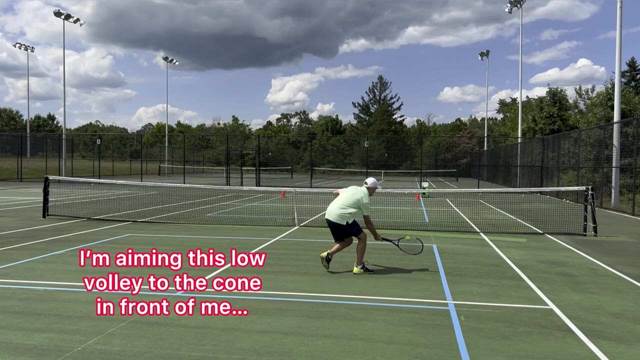 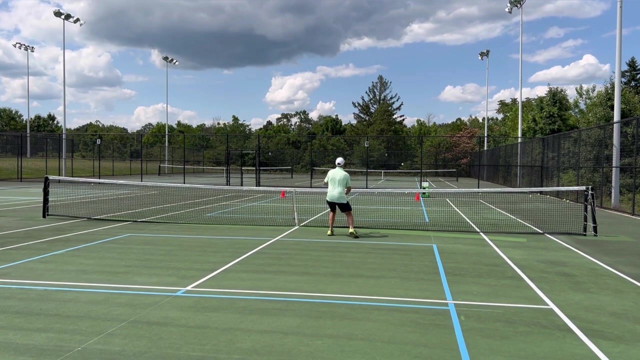 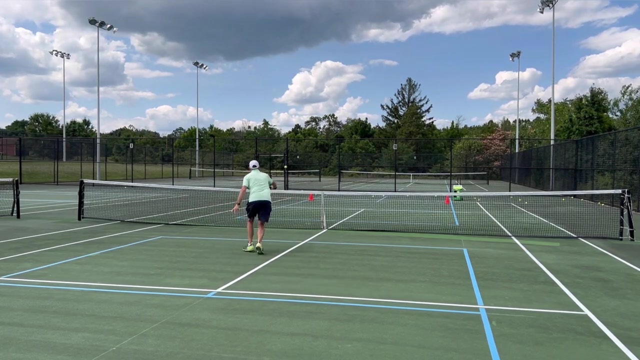 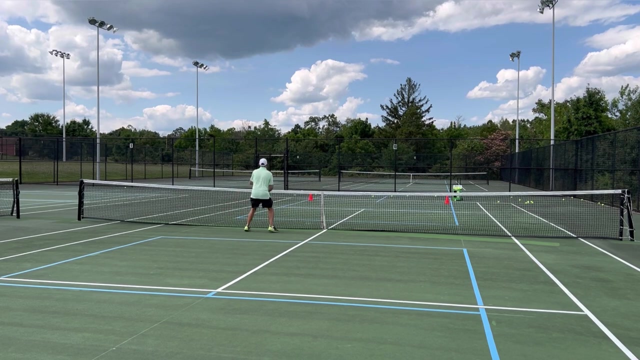 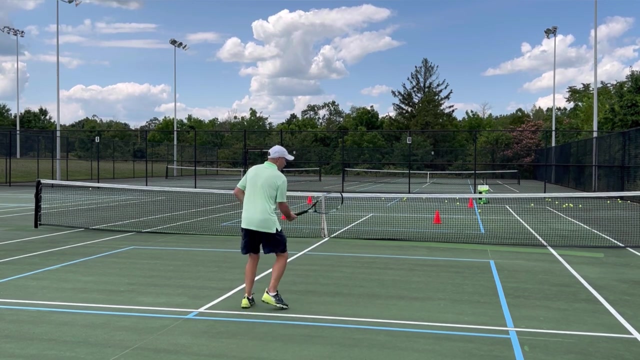 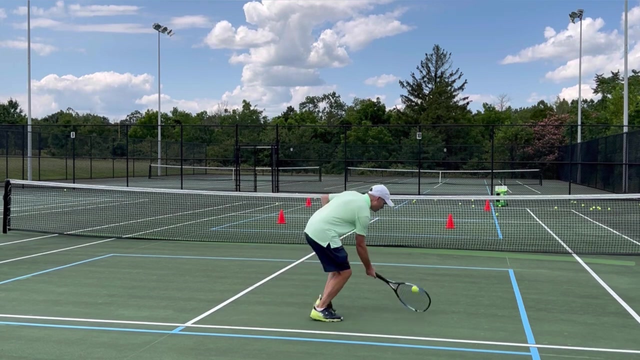 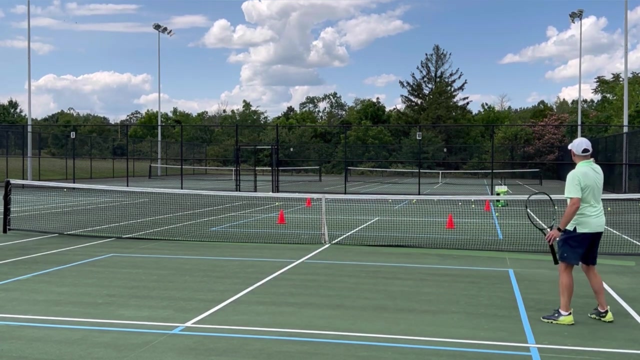 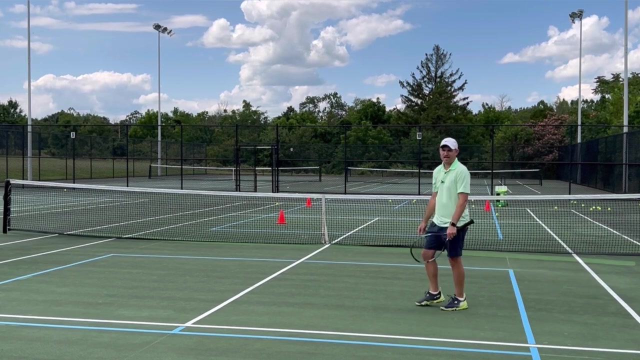 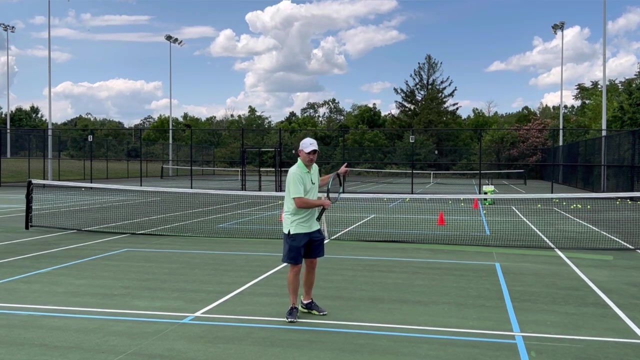 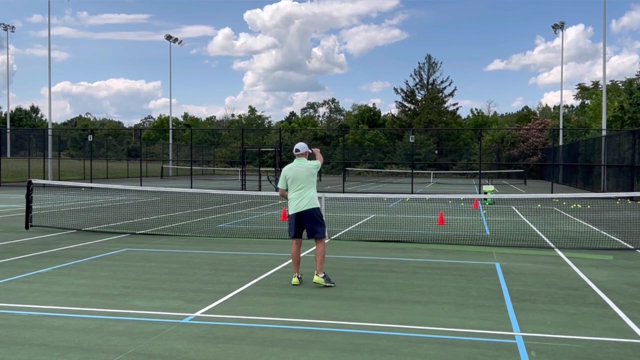 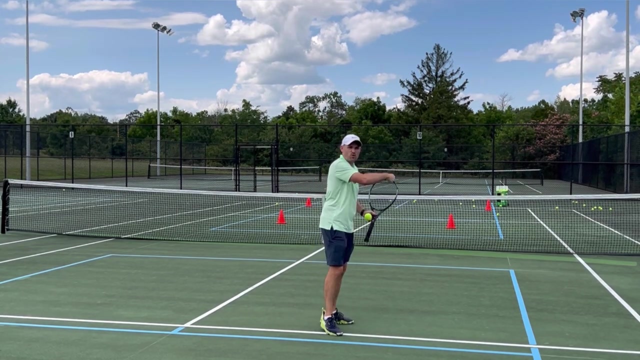 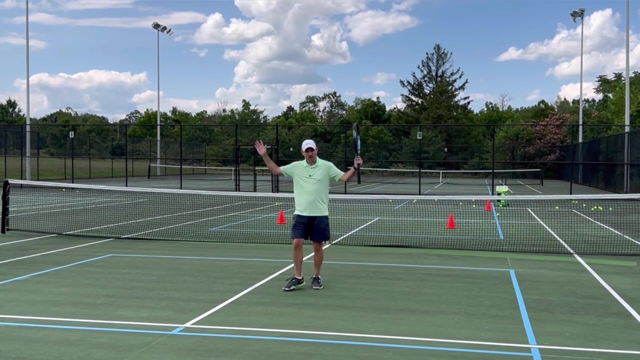 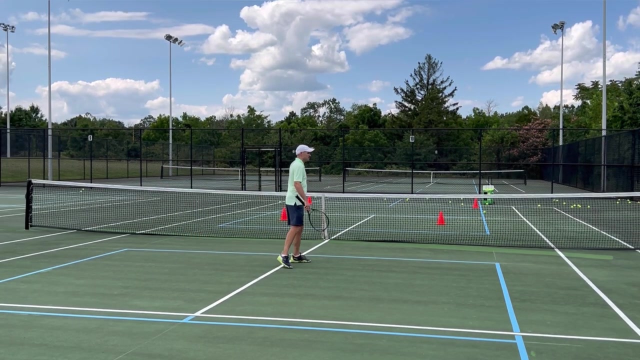 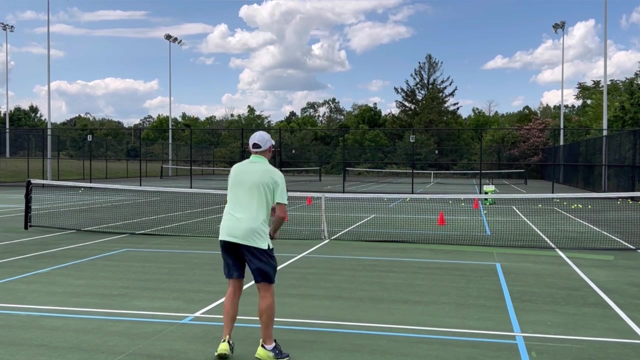 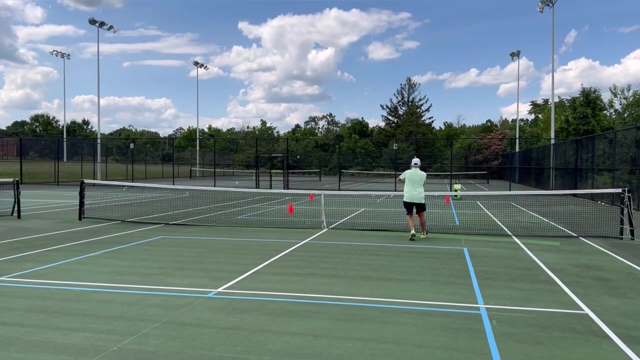 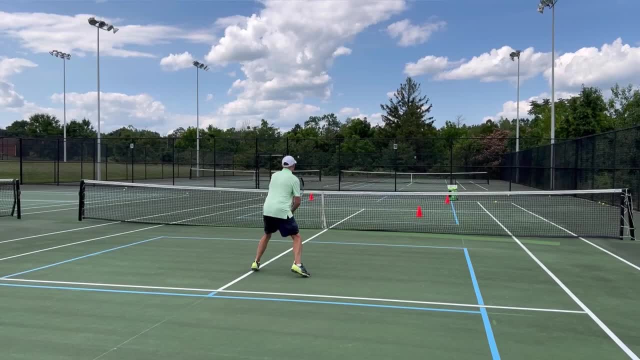 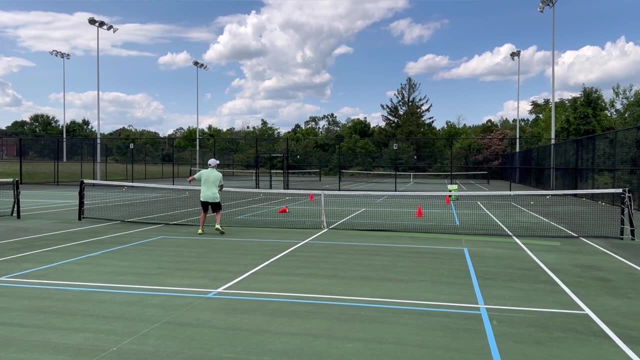 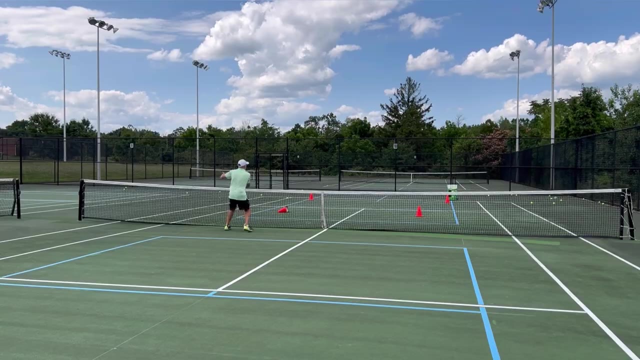 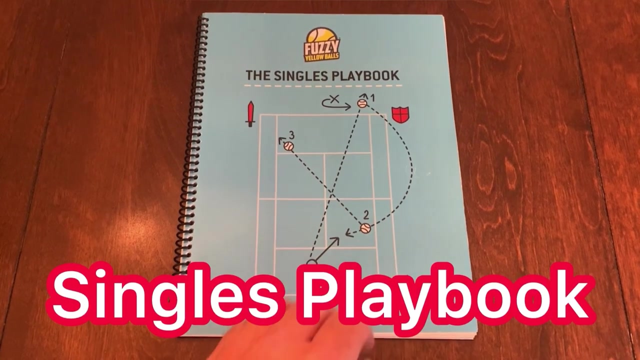 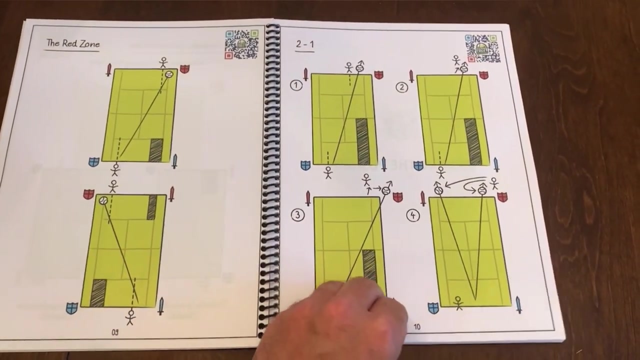 now, if you'd love to use the same strategies the pros use to win their matches, then you got to pick up the singles playbook by fuzzy yellow balls. it's all broken down by the type of opponent you play against and it's over 50 pages, strategy after strategy, and what's really cool is each.